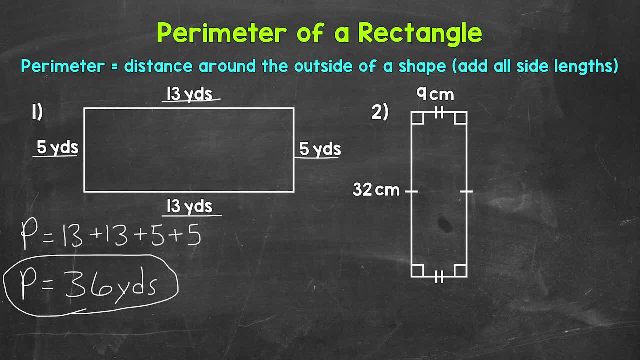 go. we can also find the perimeter by- let me write this out: perimeter equals well, multiplying the length by 2- and I'm going to use a cursive l, so it doesn't look like a 1 plus- and then multiply the width by 2.. So we can use this formula as well, just a different way to set it up. Essentially, 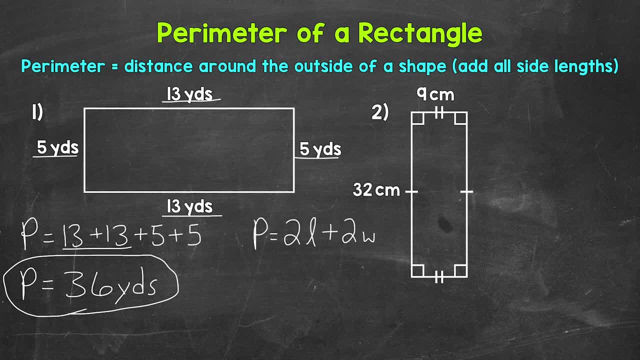 it's the same thing. You can see that we have two 13s here and then two 5s, So 2 times the length plus 2 times the width. Now I'm going to use the longer side for the length- 13- and then 5 for the width. Let's plug these in, So perimeter equals 2 times 13 plus 2 times 5.. 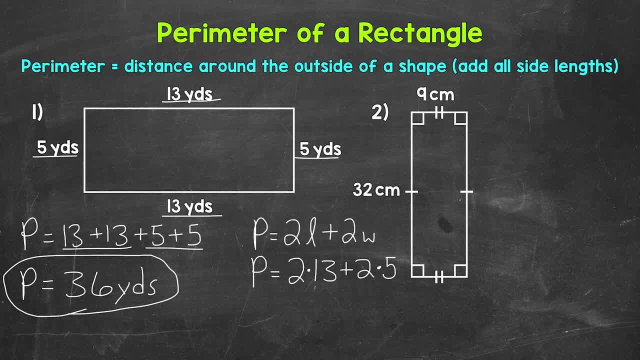 So now let's work through this and remember: we always multiply before we add. So we need to do 2 times 13 and 2 times 5.. So we need to do 2 times 13 and 2 times 5.. So we need to do 2 times 13. 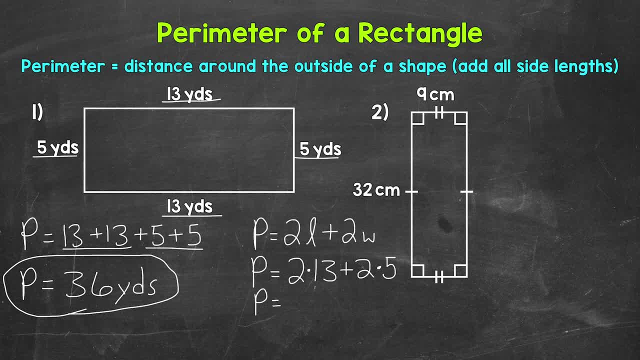 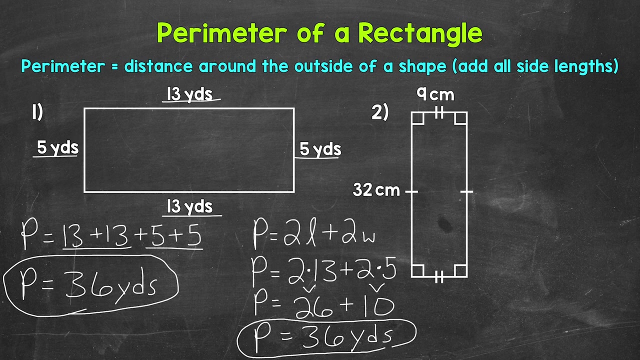 and 2 times 5.. So perimeter equals. well, 2 times 13 gives us 26, plus 2 times 5 gives us 10.. Now we can add: 26 plus 10 gives us a perimeter of 36 yards. So we get 36 yards that way as well. So for: 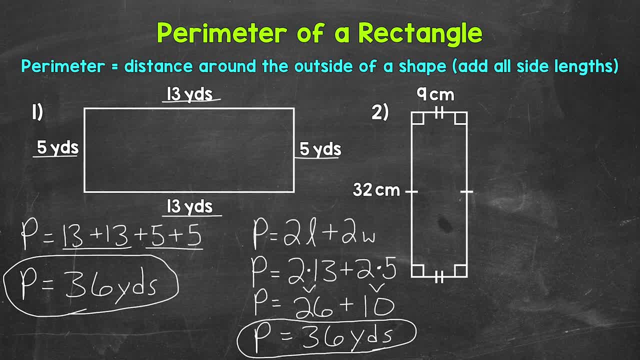 the perimeter of a rectangle. either way, we can add 26 plus 10.. So we get 36 yards that way as well. We can either add all of the side lengths or we can do 2 times the length plus 2 times the width. 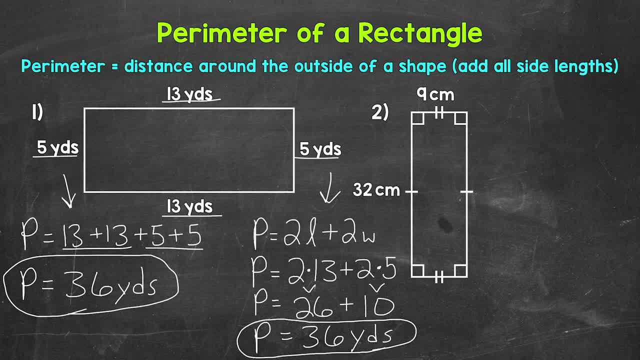 Now one more thing I do want to mention before moving on to number 2.. If we were to switch the length and the width, For example, use 5 for the length and 13 for the width, We're still going to get the correct perimeter. And for number 1, we're still going to get 36 yards. So we're going. 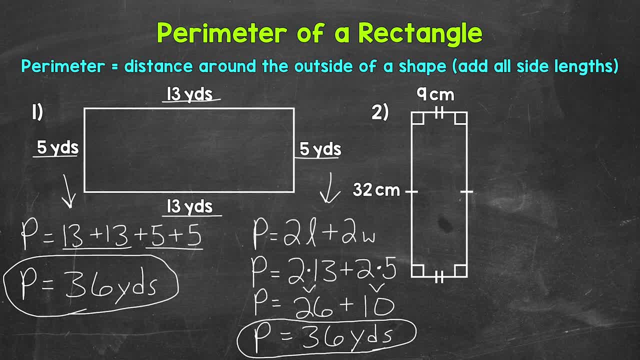 to get 36 yards. So we're still going to get 36 yards. So we're still going to get 36 yards. So don't get too held up on that. Again, I used the longer side for the length. Let's move on to. 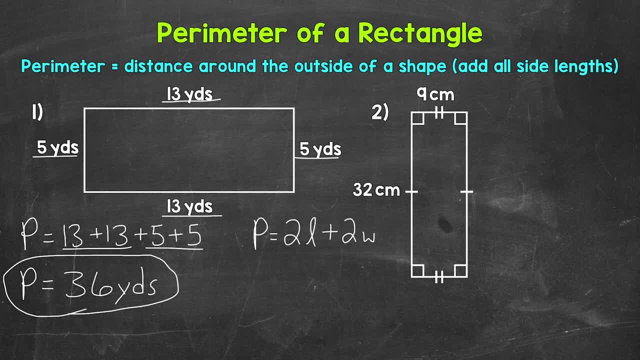 And then two 5s, So 2 times the length plus 2 times the width. Now I'm going to use the longer side for the length, 13 and then 5 for the width. Let's plug these in, So perimeter equals 2 times 13 plus 2 times 5.. 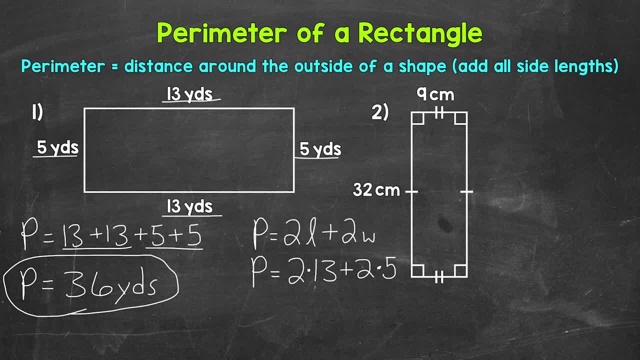 So now let's work through this And remember we always multiply before we add. So we need to do 2 times 13.. And 2 times 5.. So perimeter equals well, 2 times 13 gives us 26, plus 2 times 5 gives us 10.. 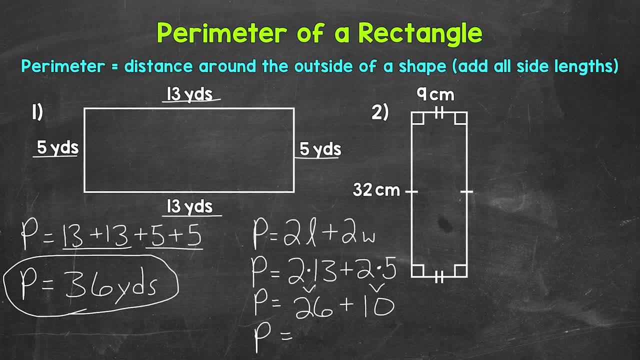 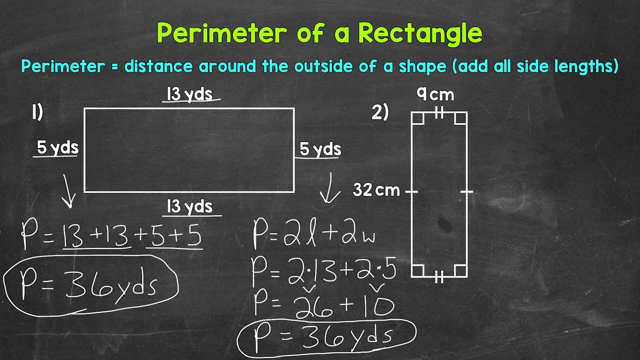 Now we can add: 26 plus 10 gives us a perimeter of 36 yards. So we get 36 yards that way as well. So for the Perimeter of a rectangle, either way will work. We can either add all of the side lengths or we can do 2 times the length plus 2 times. 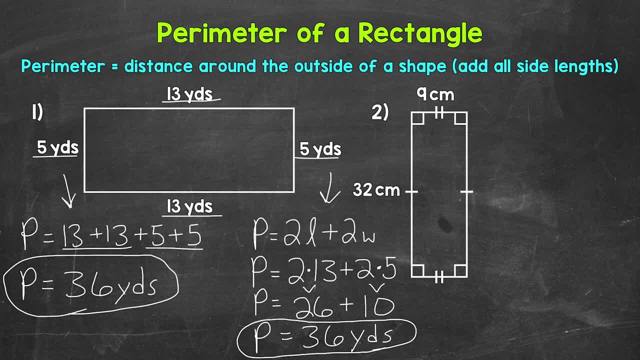 the width. Now, one more thing I do want to mention before moving on to number 2.. If we were to switch the length and the width- For example, use 5 for the length and 13 for the width- We're still going to get the correct perimeter. 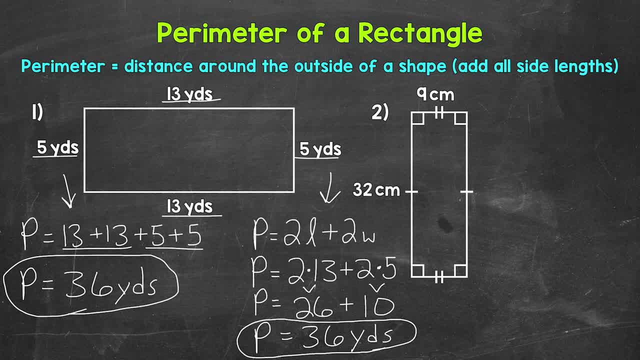 And for number 1.. We're still going to get 36 yards, So don't get too held up on that. Again, I used the longer side for the length. Let's move on to number 2 and find the perimeter of that rectangle. 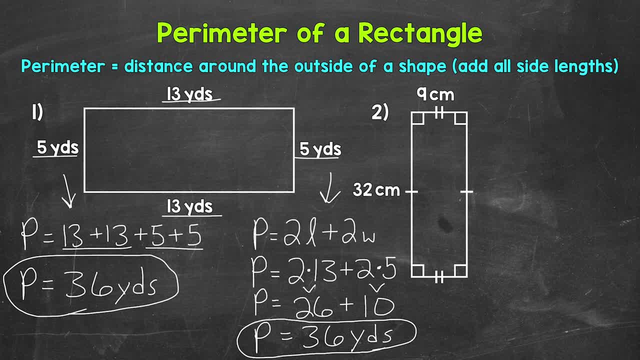 Now you'll notice that we are only given two sides. We have 32 centimeters right here and 9 centimeters right here. Well, since this is a rectangle, we know that the opposite sides are going to be the same length. So across from 32 centimeters is going to be 32 centimeters. 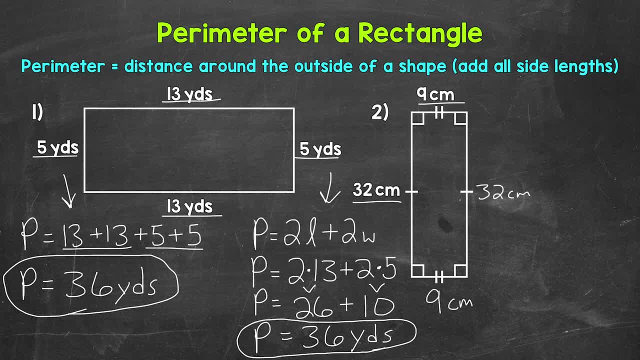 Across from 9 centimeters is going to be 9 centimeters. I also included tick marks to show this. One tick mark right here matches one tick mark right here. That shows that those sides are the same. They are both 32 centimeters. 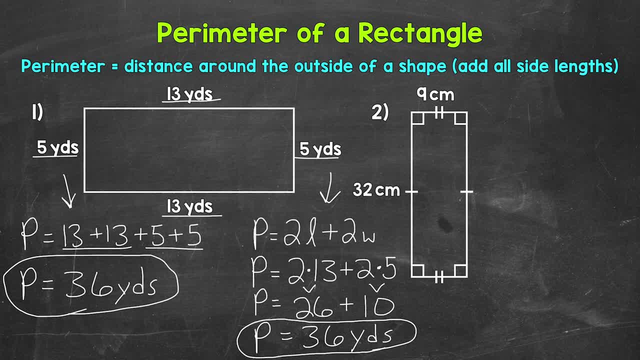 number 2 and find the perimeter of that rectangle. Now you'll notice that we are only given two sides. We have 32 centimeters right here and 9 centimeters right here. Well, since this is a rectangle, we know that the opposite sides are going to be the same length. So, across from 32. 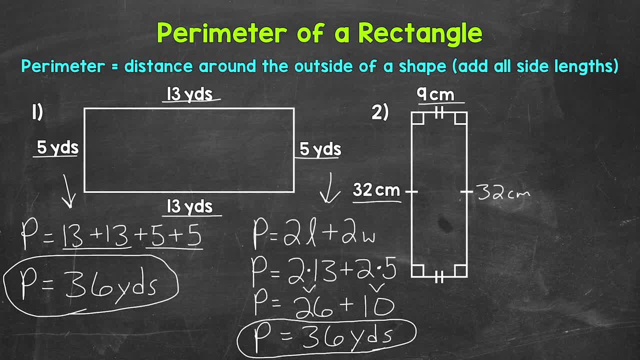 is going to be 32 centimeters Across from 9 centimeters is going to be 9 centimeters. I also included tick marks to show this. One tick mark right here matches one tick mark right here. That shows that those sides are the same. They are both 32 centimeters. And then two tick marks right here. 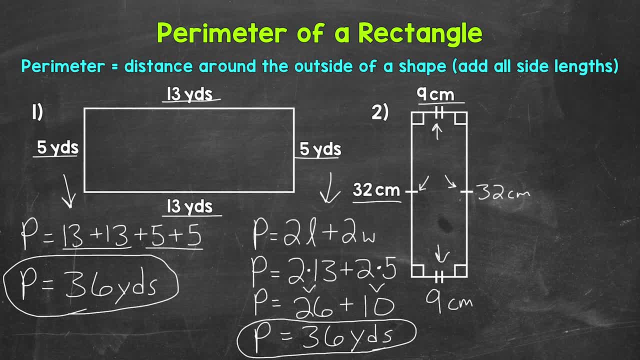 matches two tick marks right here. That shows that those sides are the same. They are both 9 centimeters. And then I also included these symbols to show that these are all right angles: 90 degree angles. I wanted to include all of these symbols in case you come across them. That way you'll know what they mean. So something. 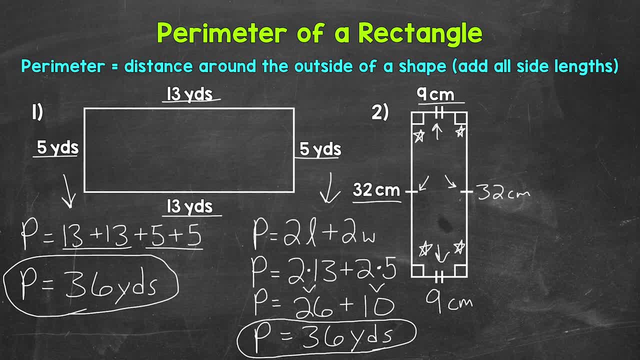 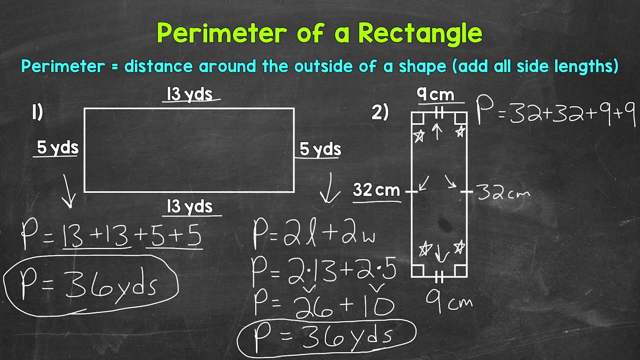 else to keep in mind. Now, as far as the perimeter, let's add all of the side lengths. So perimeter equals 32 plus 32 plus 9 plus 9.. 32 plus 32 is 64.. Plus 9 is 73.. Plus 9 is 82. So we have a. 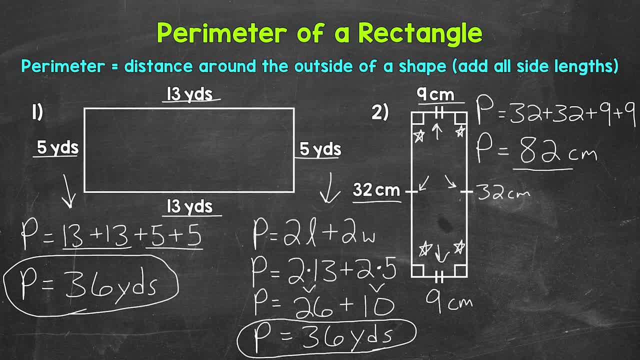 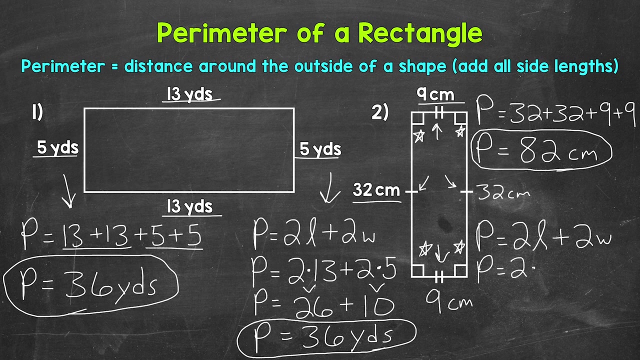 perimeter of 82 centimeters. Now let's also multiply the length by 2 and the width by 2.. then add those, so let's do it that way as well. so perimeter equals two times the length plus two times the width. let's use 32 for the length, so 2 times 32 plus. 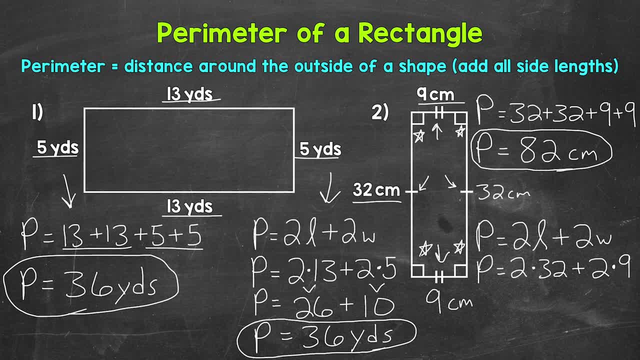 and then 9 for the width, so 2 times 9.. let's multiply now: 2 times 32 is 64 plus 2 times 9 is 18.. 64 plus 18 gives us a perimeter of 82 centimeters, so we get the same. 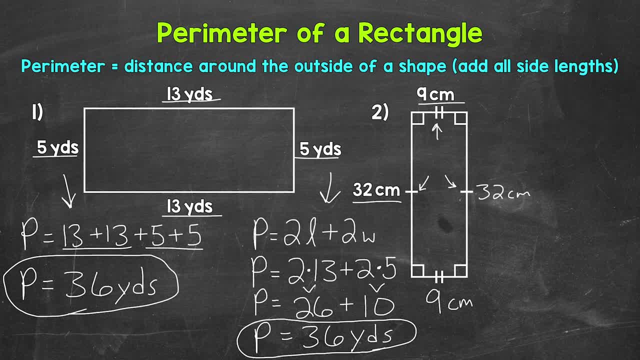 And then two tick marks right here: match, Right here matches. two tick marks right here showing that those sides are the same. They are both 9 centimeters. And then I also included these symbols to show that these are all right angles: 90 degree. 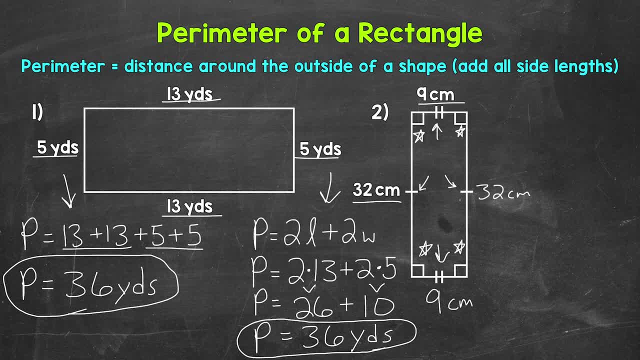 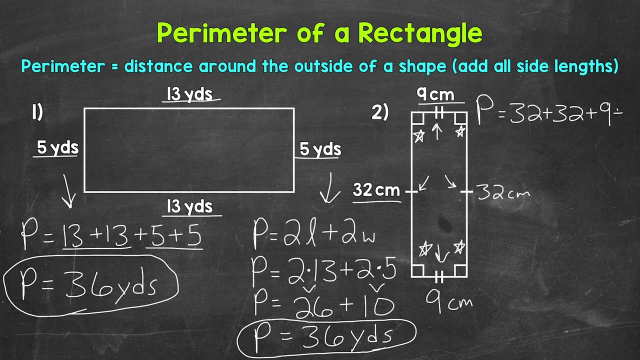 angles. I wanted to include all of these symbols in case you come across them. That way you'll know what they mean. So something else to keep in mind. Now, as far as the perimeter, Let's add all of the side lengths, So perimeter equals 32 plus 32 plus 9 plus 9.. 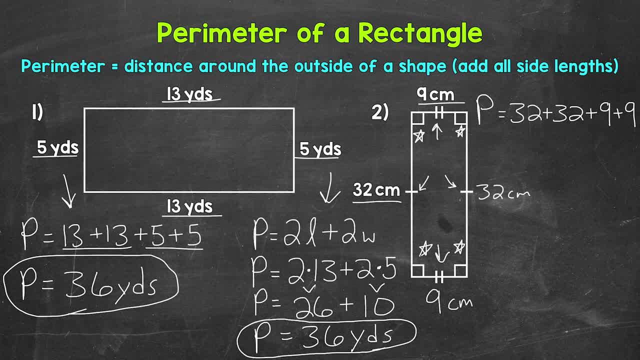 32 plus 32 is 64, plus 9 is 73, plus 9 is 82. So we have a perimeter of 82 centimeters. Now let's add the side length. Now let's also multiply the length by 2 and the width by 2 and then add those. 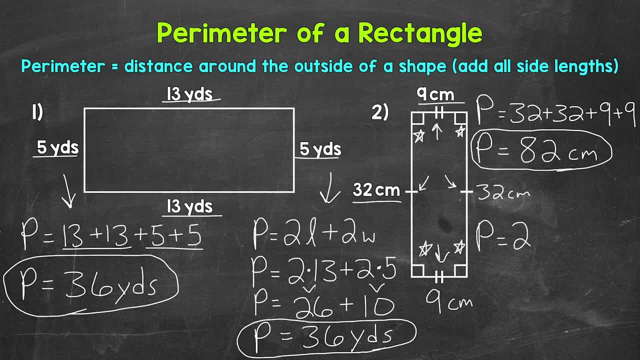 So let's do it that way as well. So perimeter equals 2 times the length plus 2 times the width. Let's use 32 for the length, So 2 times 32 plus, and then 9 for the width, So 2 times 9.. 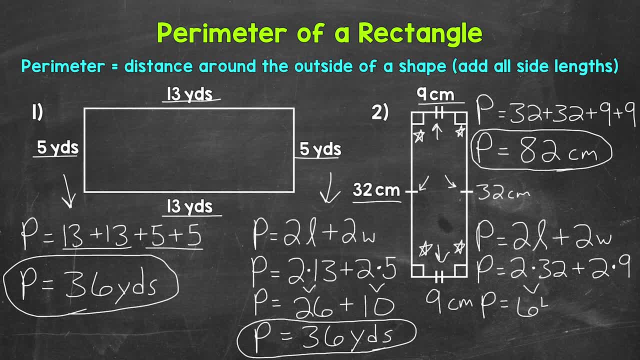 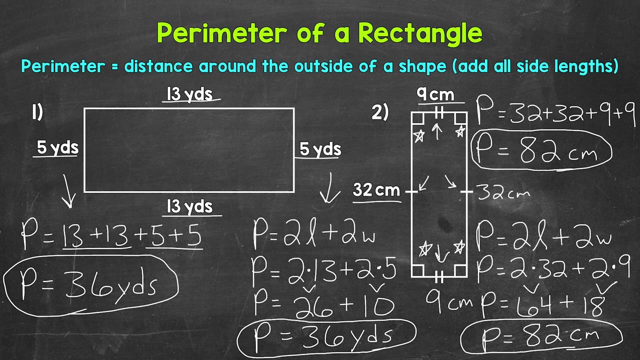 Let's multiply now: 2 times 32 is 64 plus 2 times 9 is 18.. 64 plus 18 gives us a perimeter of 82 centimeters, So we get the same perimeter that way as well. Now again, I do want to mention I used the longest side for the length in both of these. 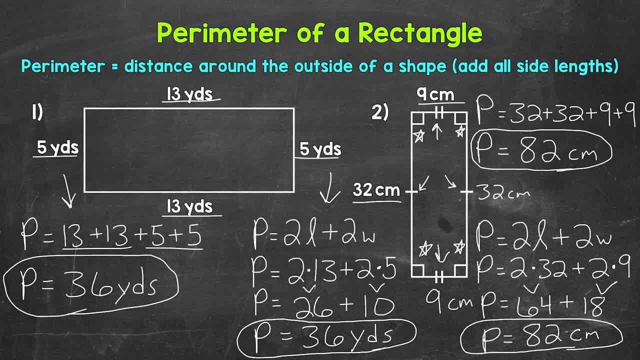 examples. If we do switch up the length and the width, We're still going to get the correct perimeter. So don't get too held up on which is the length and which is the width. If you want to keep it consistent, just go with the longest side for the length. 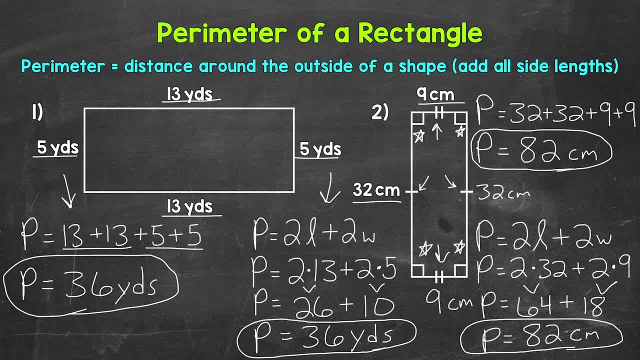 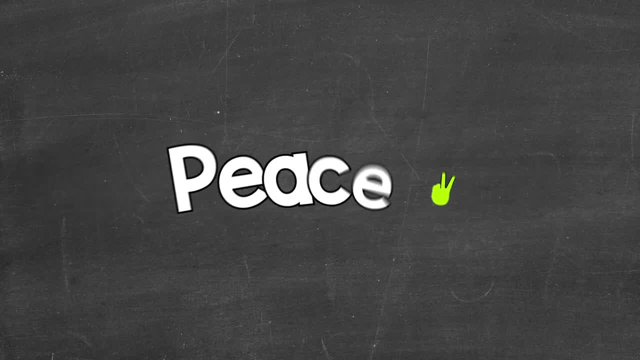 So there you have it. There's how to find the perimeter of a rectangle. I hope that helped. Thanks so much for watching. Until next time, Peace, Peace, Peace.